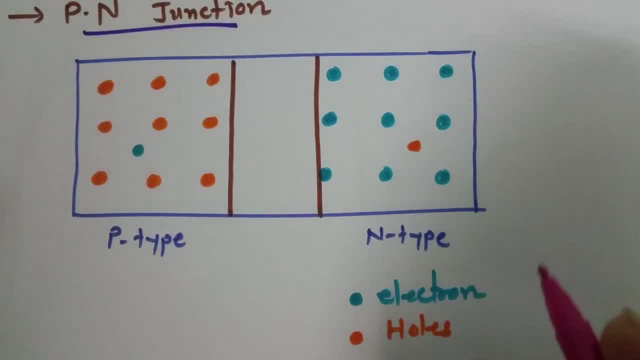 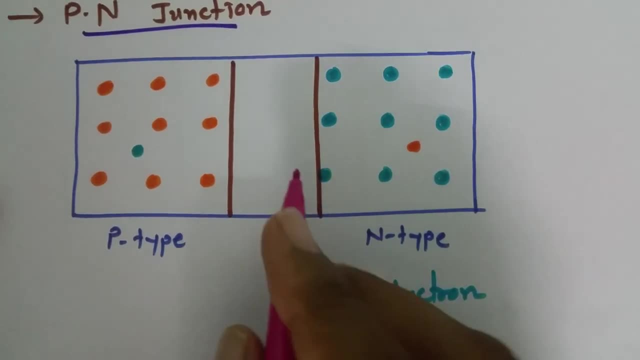 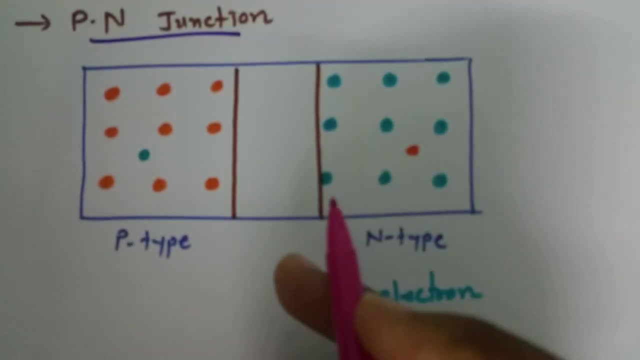 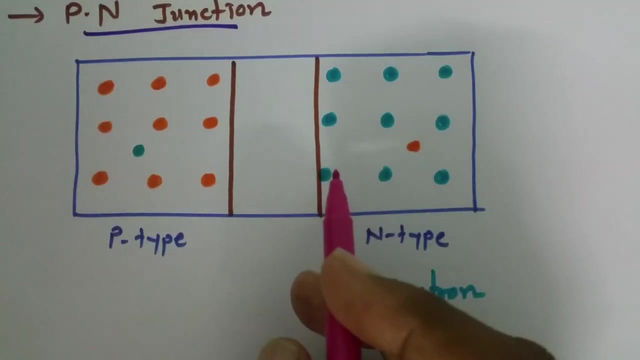 due to pentavalent impurities are added inside, and now if we diffuse p-type and n-type material together, it is forming pn junction. so when we diffuse together, some electrons from n-type material are getting combined with p-type materials holes and that is forming ion. so 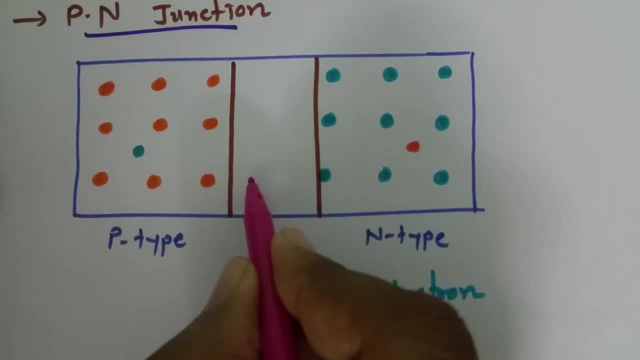 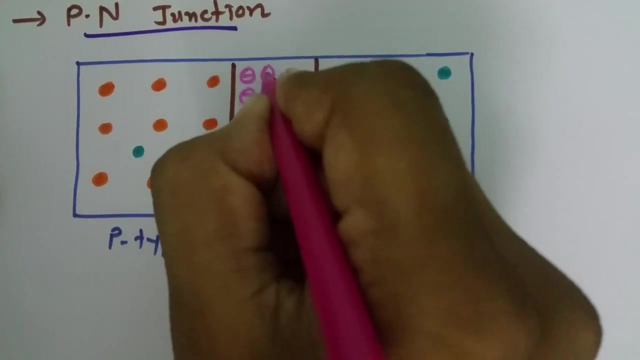 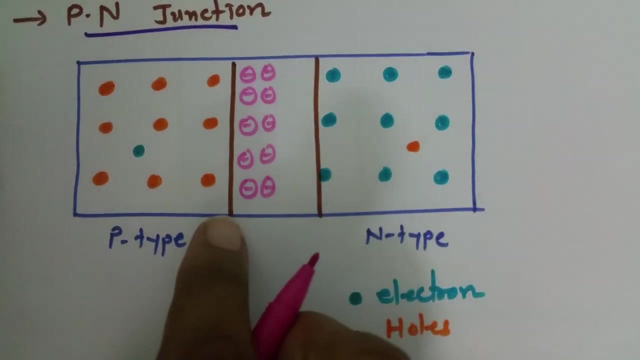 what happens is like at p-type material there are holes and that is getting combined to electrons of n-type material and that forms negative ion over this side. so when we diffuse p-type and n-type material, it forms negative ions at the side of p-type material and at n-type material. 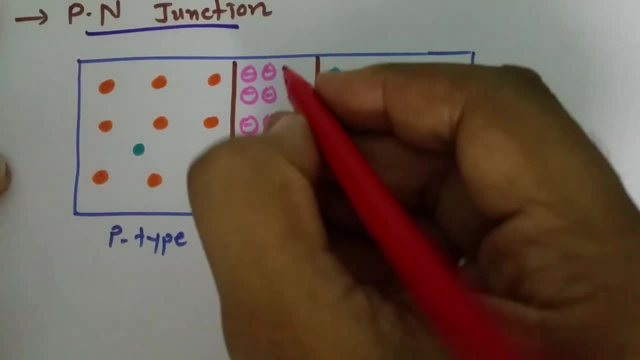 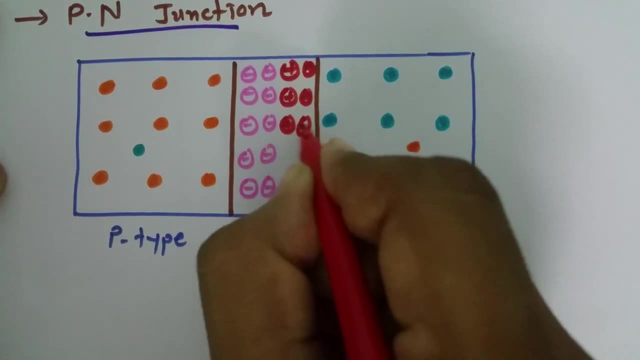 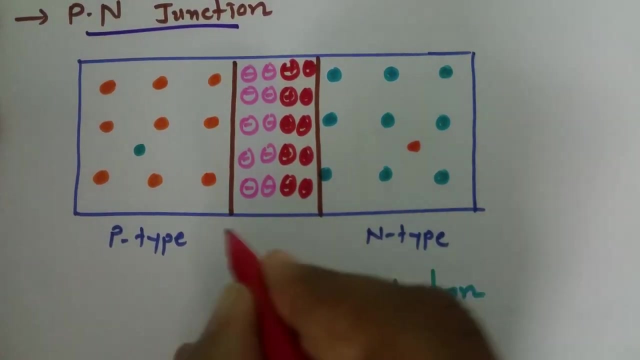 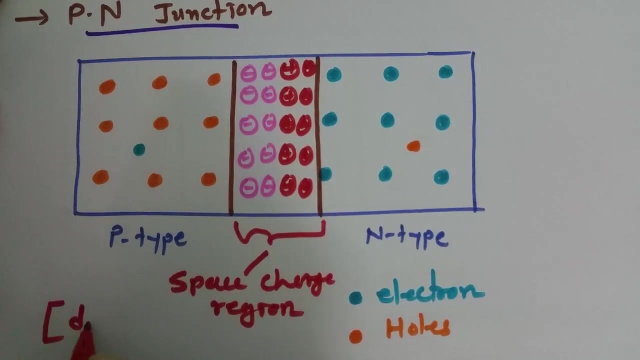 holes are getting combined with electrons and that forms positive ions. so here we can observe positive ions because of diffusion of p-type and n-type material and this region is called as space charge region, or even it is called as p-type material, called as depletion region. So this region is called as phase charge region, or even we. 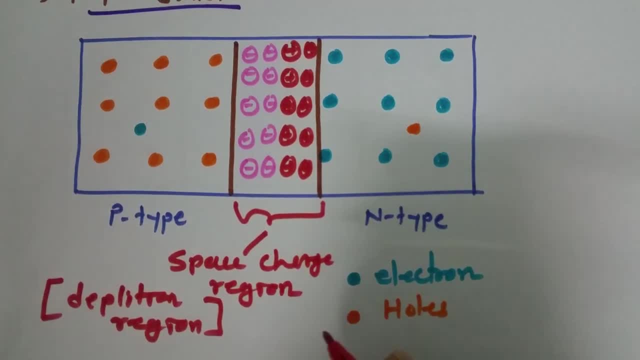 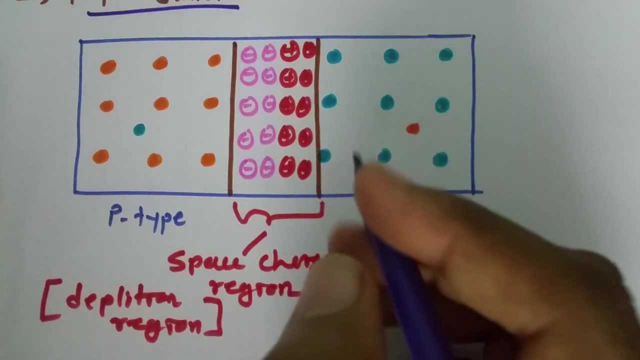 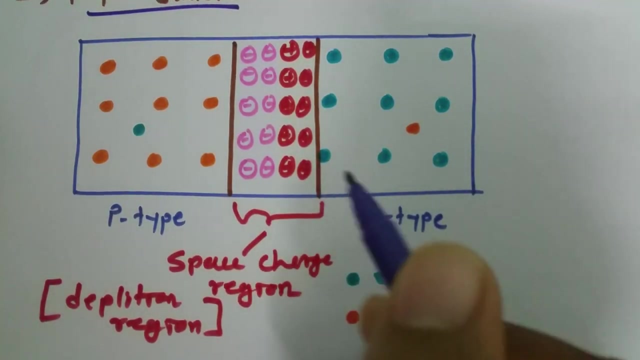 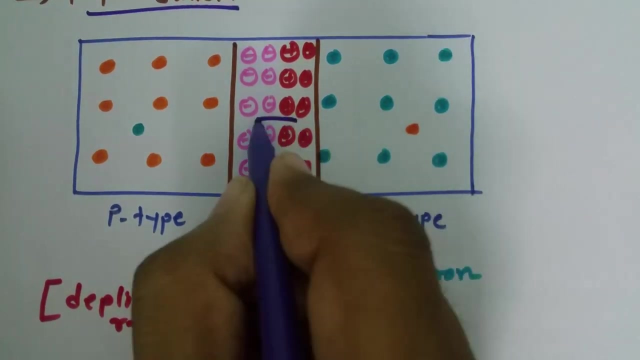 can say this region is even called as a depletion region. Now over here electrons are there in n type material and holes are there with p type material and at phase charge region. some holes are there at n type material, are moving towards this and some electrons 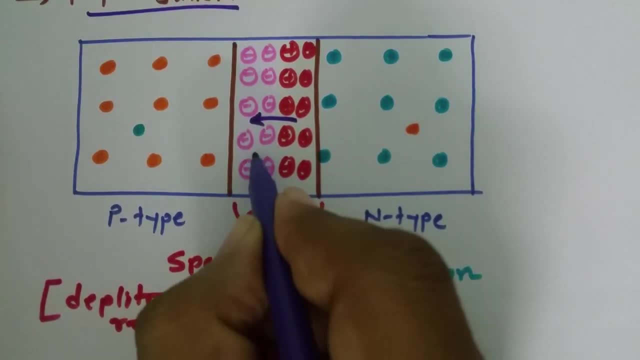 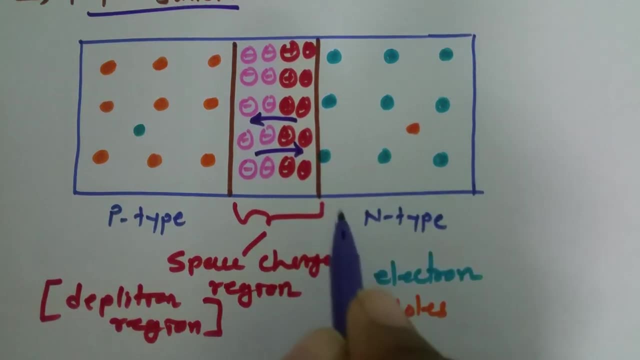 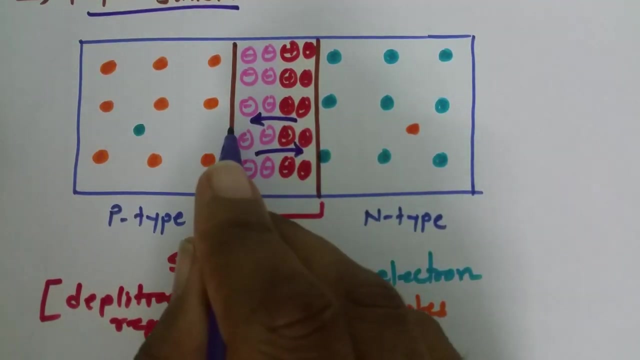 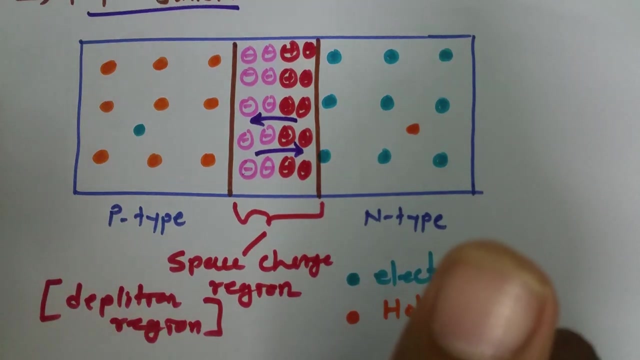 which are there over here in negative ion. those are moving towards this. So electrons are moving from p-type material to n-type material at space charge region and holes are moving from n-type material to p-type material in space charge region and that will move continuously till equilibrium is happening and because of that motion of charges current. 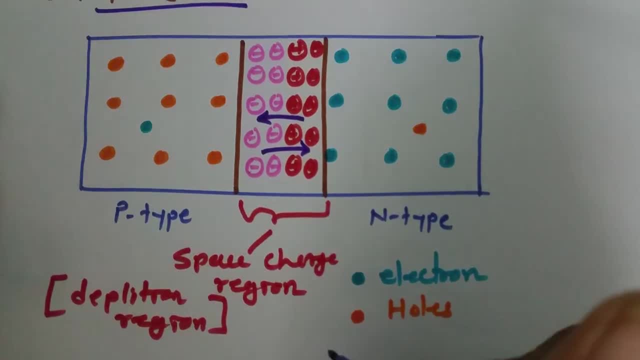 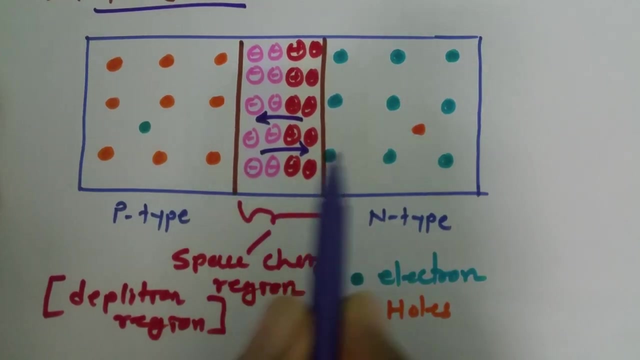 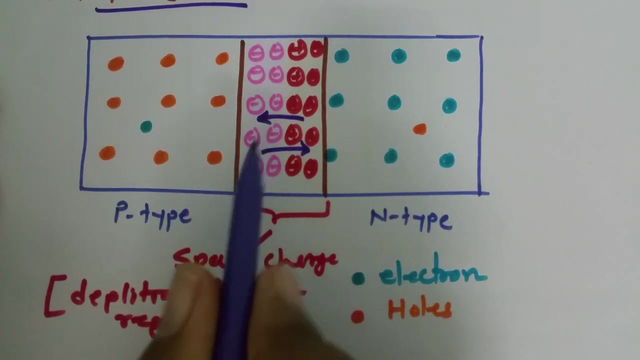 flows and that current is called as diffusion current. So see, ultimately, when we diffuse p-type and n-type material together at a junction, p-type materials- holes are getting combined with n-type materials. electrons at p side resulted into negative ions and at n side it will resulting into positive ions, even though those there 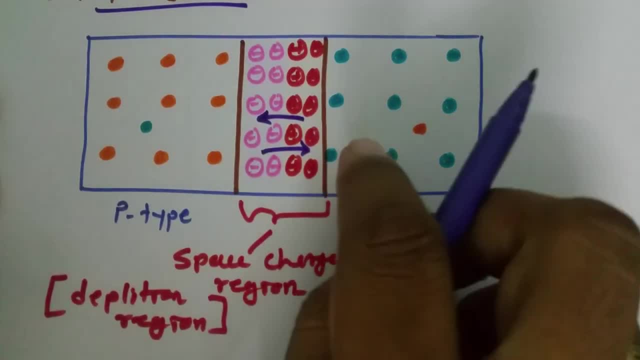 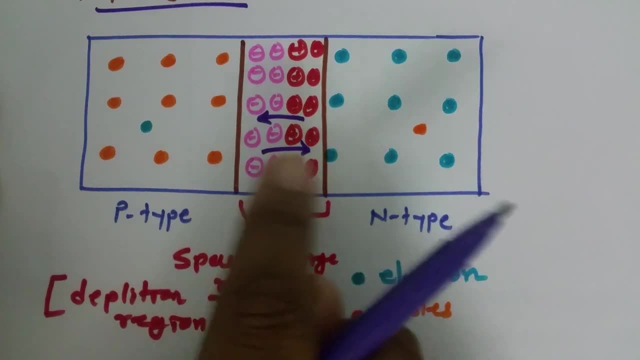 are ions. holes at the side of p-type material are moving towards p-type material and electrons at the side of p-type material are moving towards n-types material, and that will move till equilibrium happens. So there is no change in the current of the radioactive charge, which is the current. 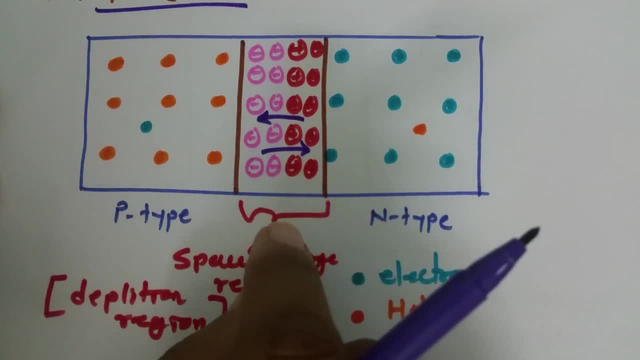 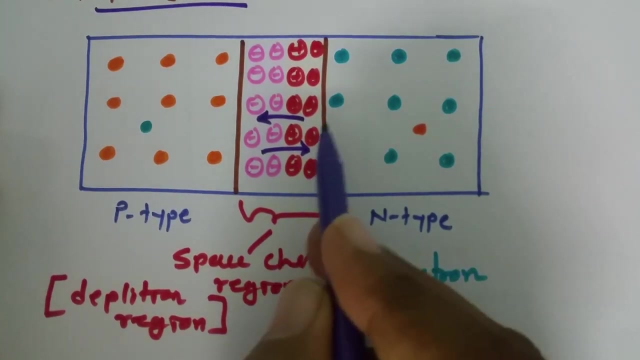 that is just coming from the p-type materials And that charges are resulting into flow of current and that flow of current is called as diffusion current. So that is happening because of diffusion of electrons and holes which is happening at junction. that is why that current is called as diffusion current and when diffusion is. 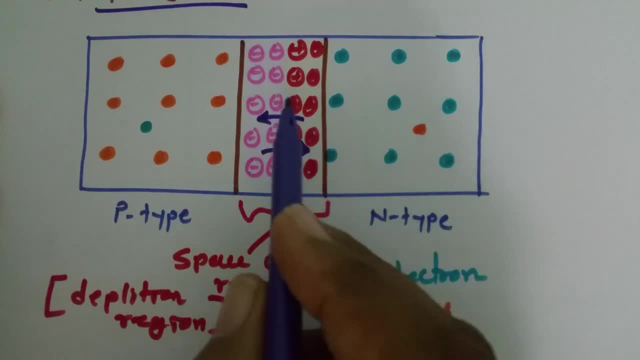 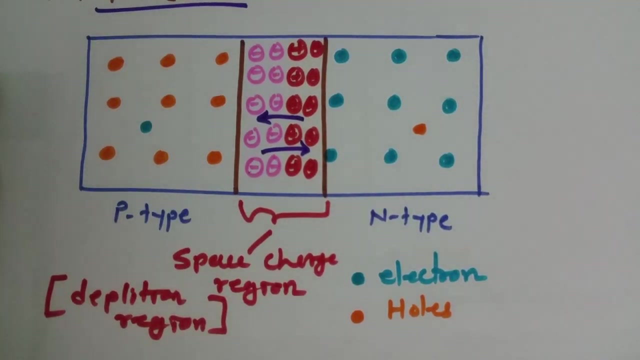 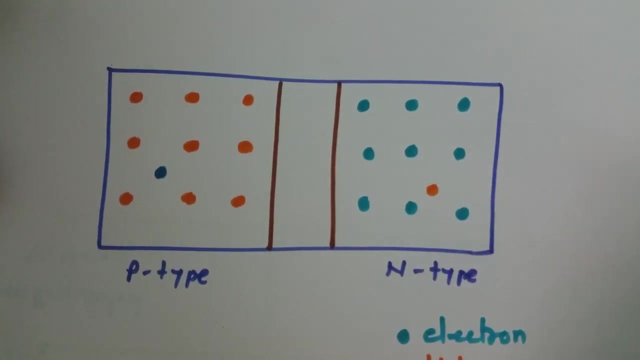 happening. at junction, ions are generated, So this is also called as diffusion current. at junction, those ions region is called as depletion region or space charge region. Now let us try to understand p-n junction in forward bias. So here I am connecting. 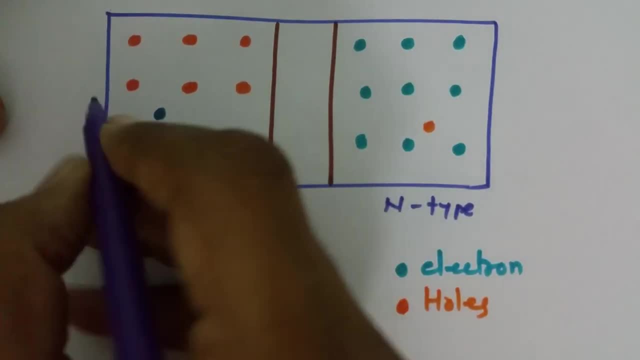 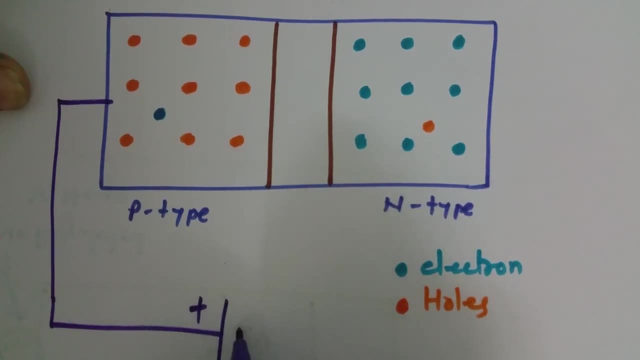 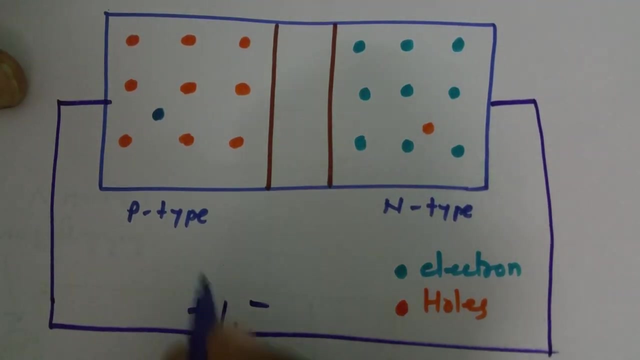 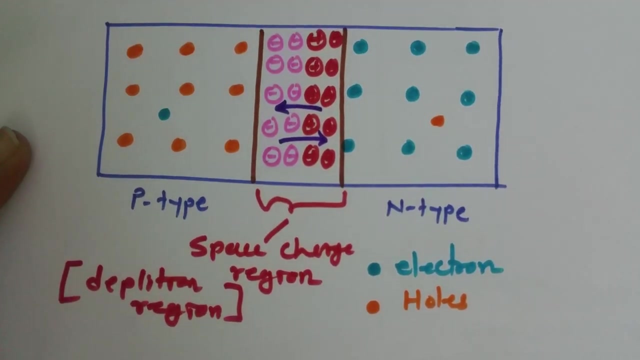 this p-n junction in forward bias. So if I connect p-type material with positive terminal of battery and n-type material with negative terminal of battery, then this p-n junction will come in forward. bias comes in forward bias depletion region when it was not biased at the time. it 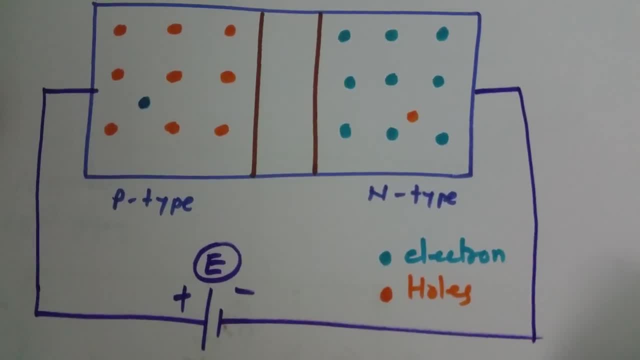 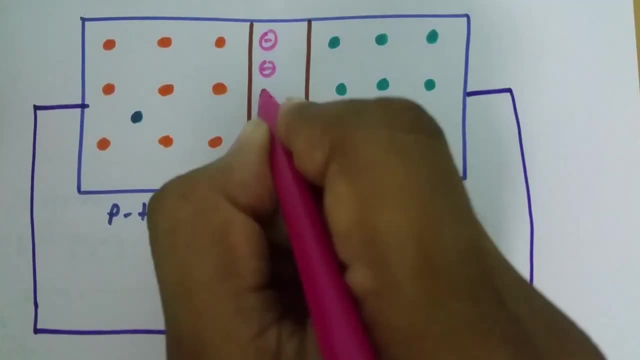 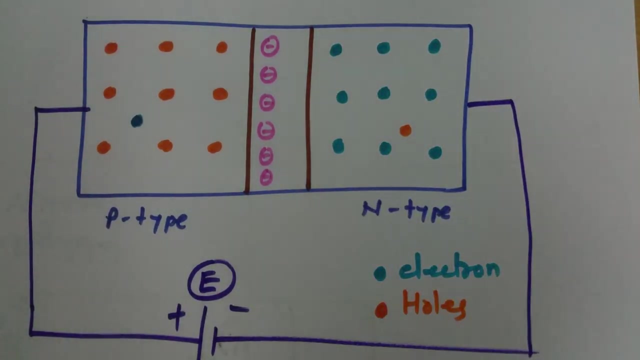 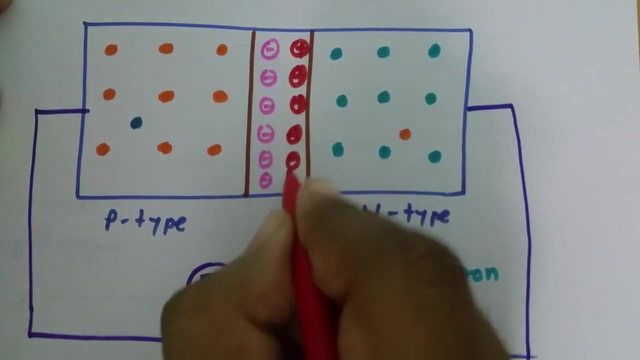 was this much. but once you connect that to forward bias, that depletion region will decrease. so right now we can see negative ions, which is there at p-type material, and positive ions- these are there in the side of n-type material- and that region is depletion region. so that depletion region is getting contracted. 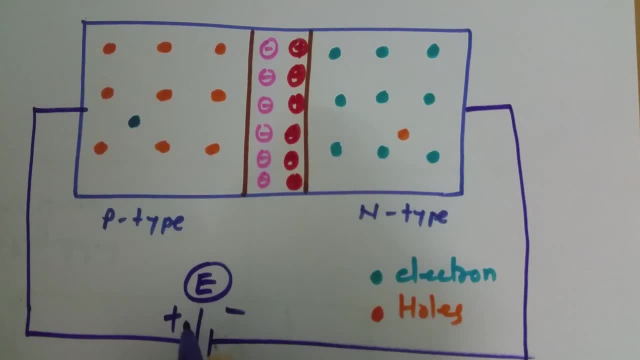 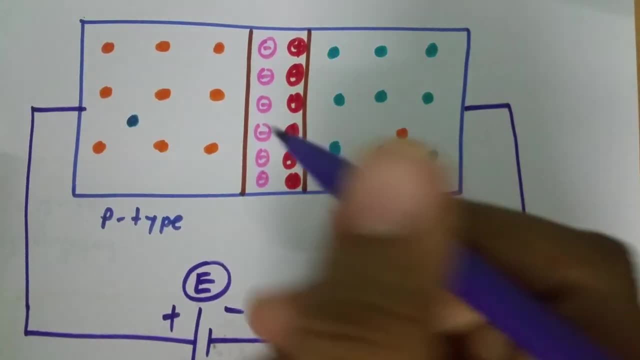 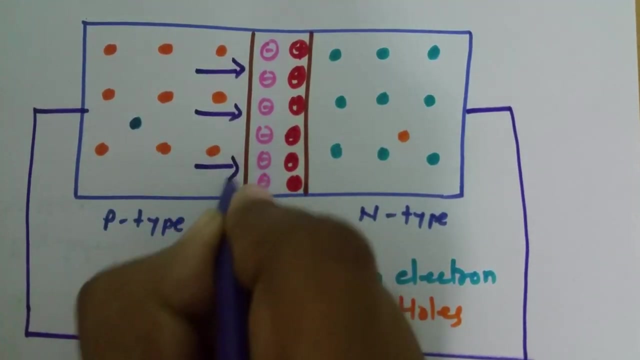 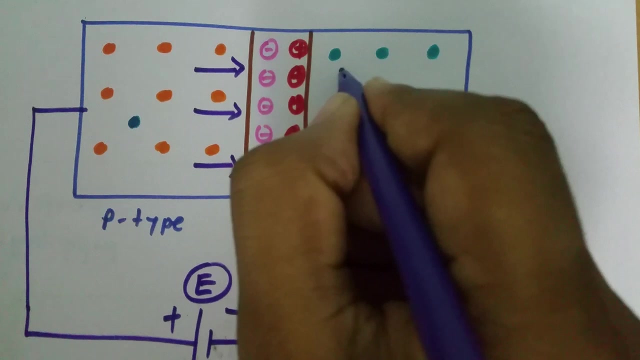 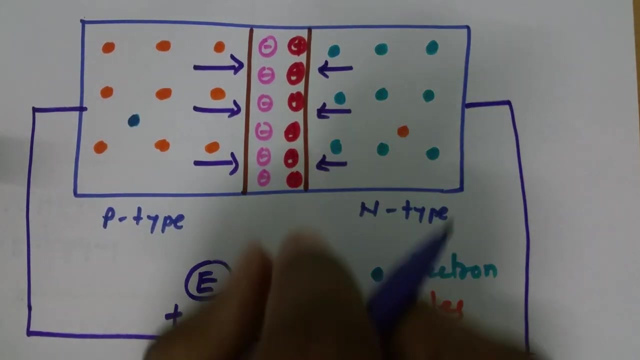 and that contraction that happens because of when we connect positive terminal of battery to p-type material, those holes which are there towards p-type material that is giving pressure on this region, like this, and negative terminal of battery is connected to n-type material that is giving pressure to depletion region, like this. so, ultimately, because of this, 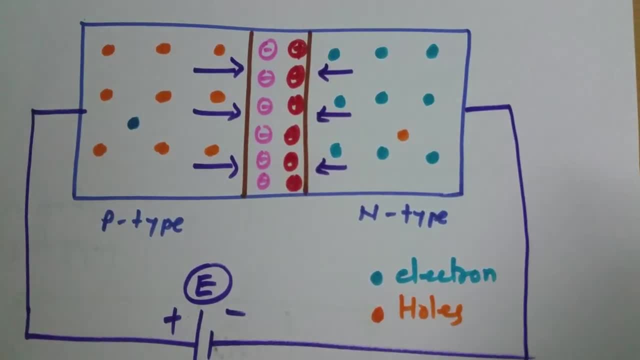 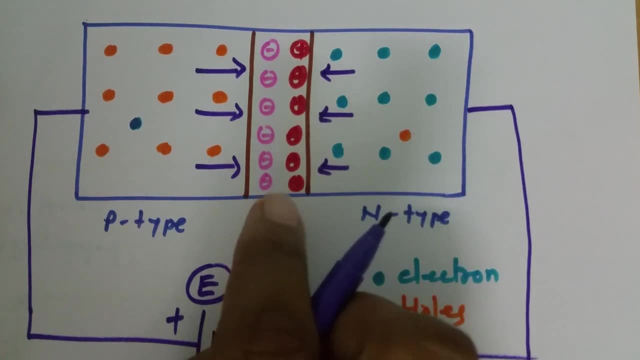 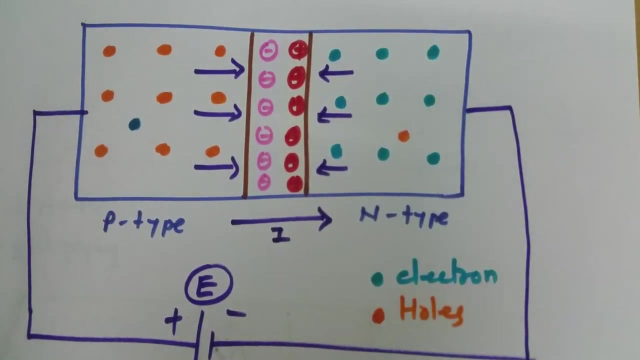 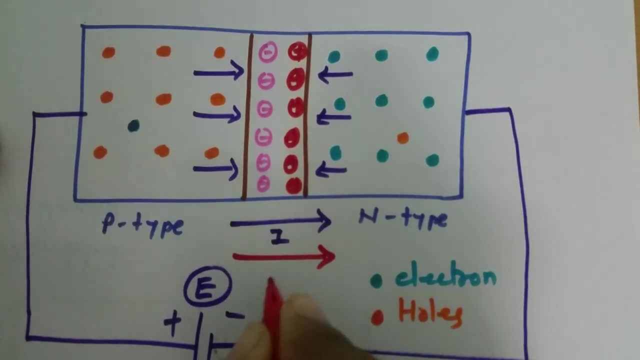 pressure on depletion region. this depletion region is getting contracted and after we give potential barrier amount of potential, it will start to conduct so conventional, current direction that will be in this direction. this will be the direction of current and the direction of holes that will be in this direction. so this will be the 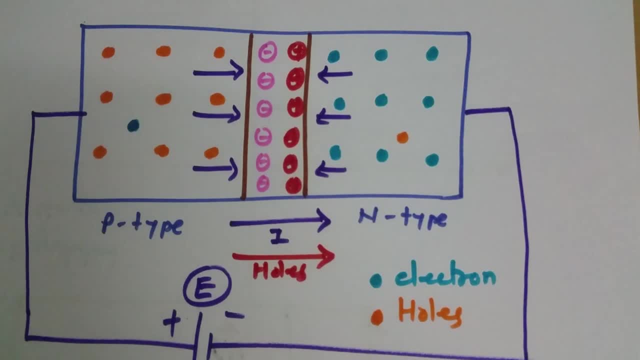 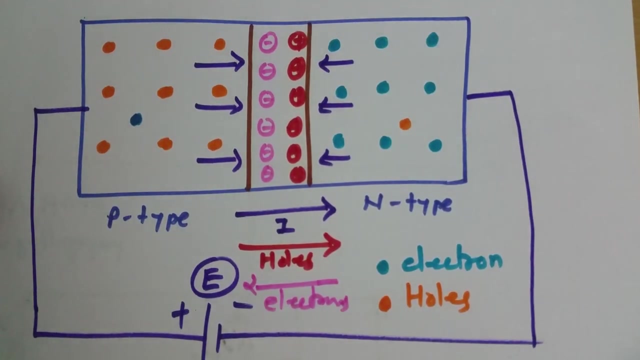 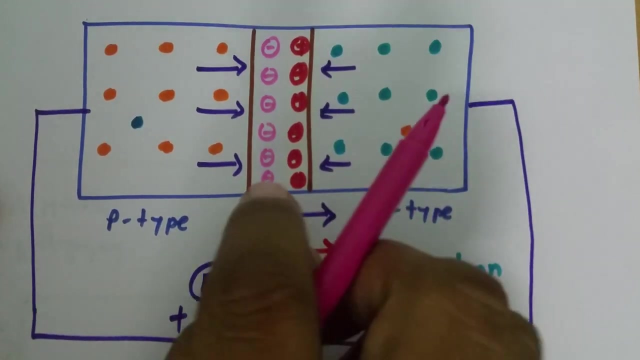 direction of holes and the direction of electrons that will be in the direction opposite to the direction of flow of current. so this will be the direction of electrons. so that is how complete flow of current happens. and when current flows by contracting this depletion region, that current is called as drift. 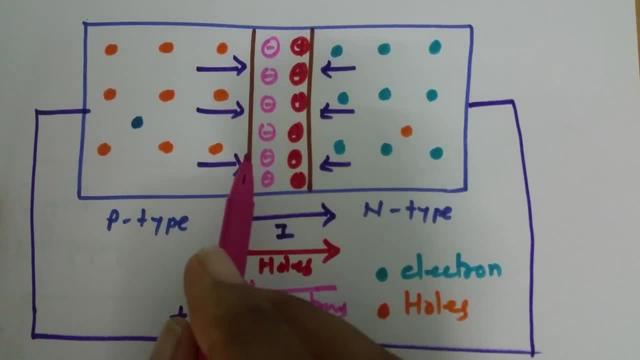 current. the reason is this: current is happening because of drifting of charges from p-type to n-type as holes and from n-type to p-type as electrons, so those drifting of charges that happens because of this potential which is connected in forward bias to this p-n junction, so that current is called as a drift. 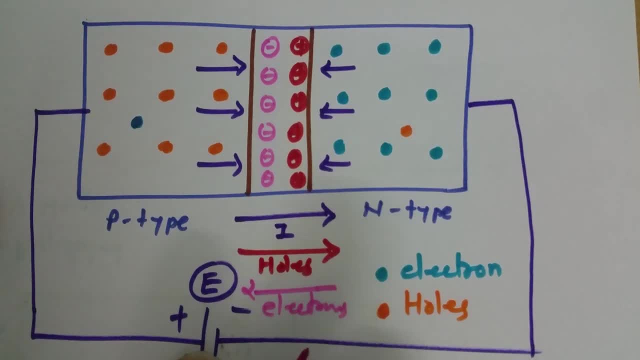 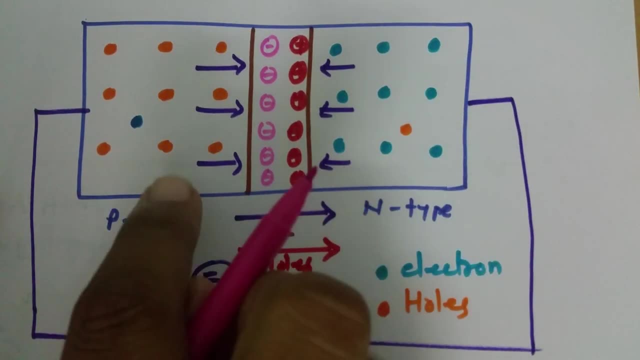 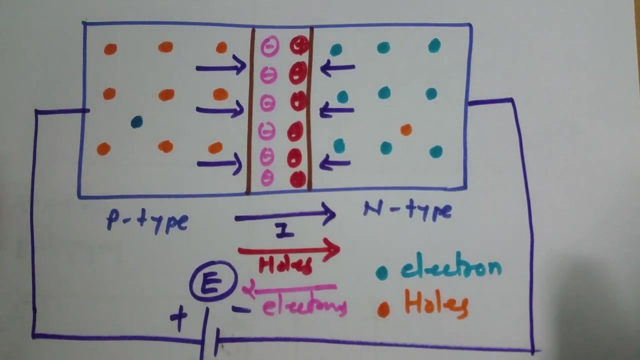 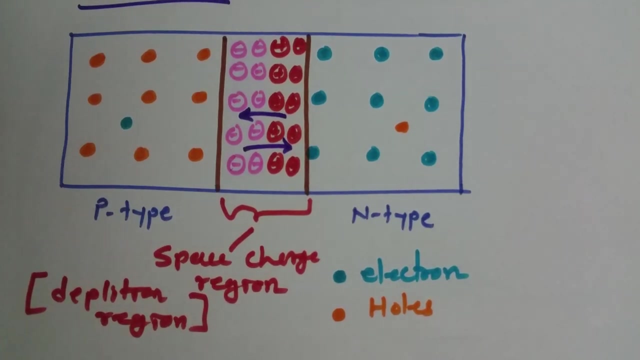 current. so drift current, that happens because of battery connected to p-n junction and that battery is resulting into drift of holes from p-type to n-type and drift of electrons from n-type to p-type. so that is how drift current is happening. now, again, let us see this p-n junction. so here, when we see this p-n. 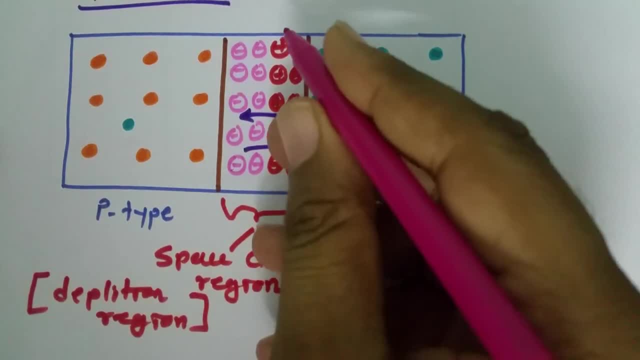 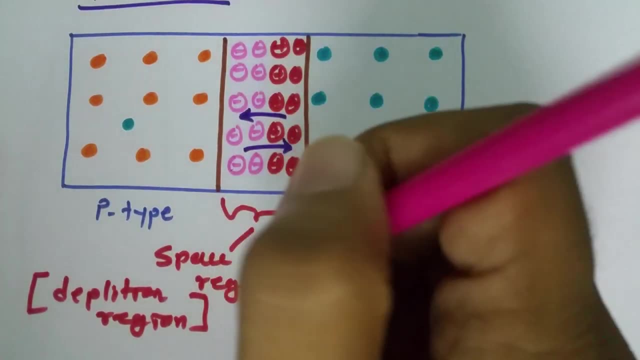 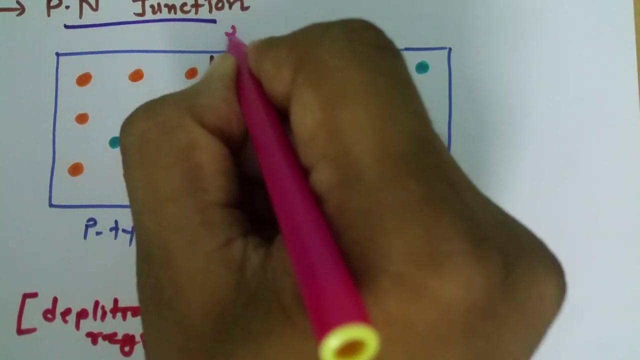 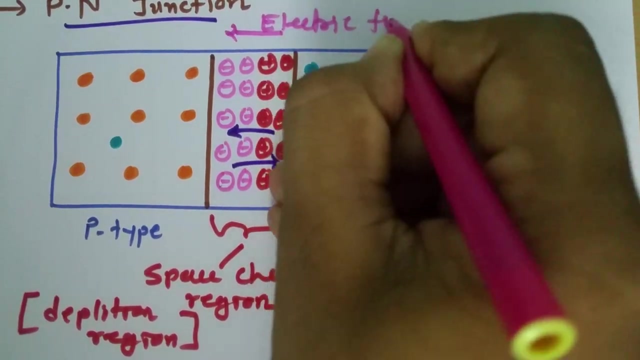 junction. here there are positive ions, which is getting resulted at the side of n-type material, and negative ions, that is resulted at the side of p-type material. so that is resulting into electric field and that electric field direction that will be from positive ions to negative ion. so this electric field will be in the direction from n-type. 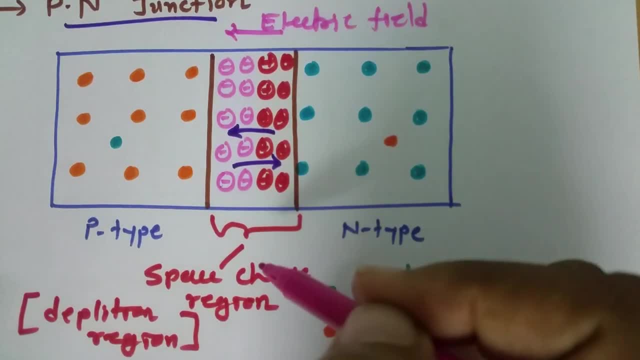 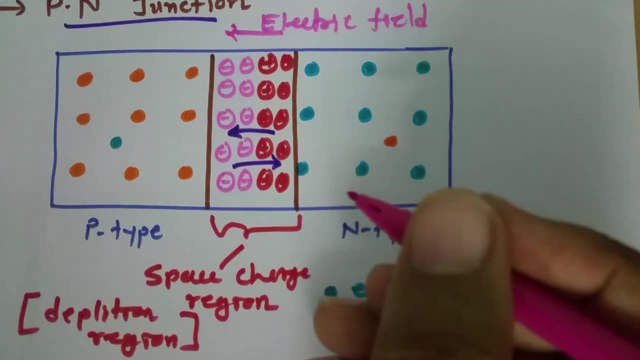 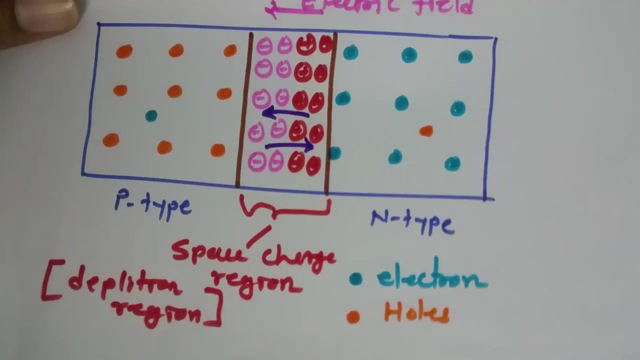 material to p-type material. the reason is: positive ions are getting generated at the side of n-type material and negative ions are getting generated at the side of p-type material. so now again, let us move back to reverse bias characteristic so that we can understand how exactly that functions. 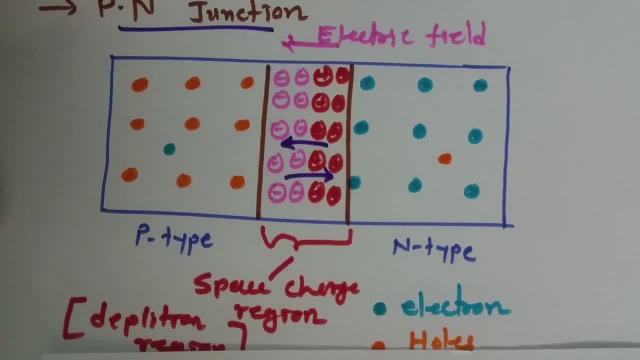 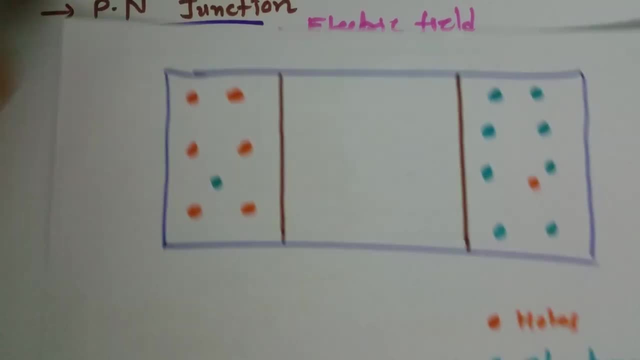 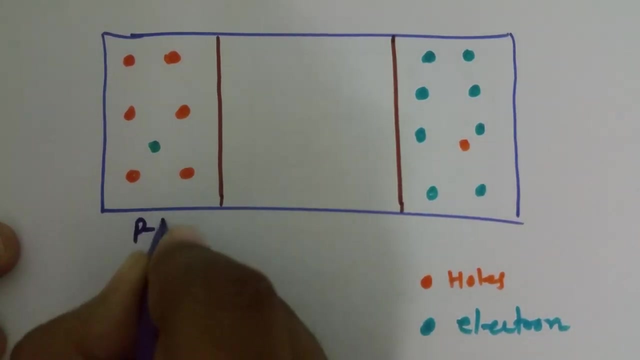 so before we plot out forward bias and reverse bias characteristic, let us try to understand what if we connect p-n junction in reverse bias, so, as we can see here, this is p-type material and this is n-type material that is connected to a future phase. before we plot out forward and reverse bias characteristics and we see this is a p-type material and this is un-type material that is connected to an aren two members. so that means and n-type material is connected to a n-type basis. so we have 2 options. that is you can see in this scheme. so we can see injuries PER. If P'n equates P'n equal to Gulb & N smaller than, yes, P'n срав ro, it may be enough for that capture. this can be saved. 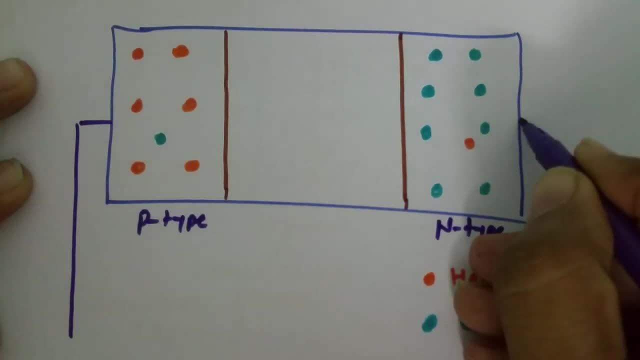 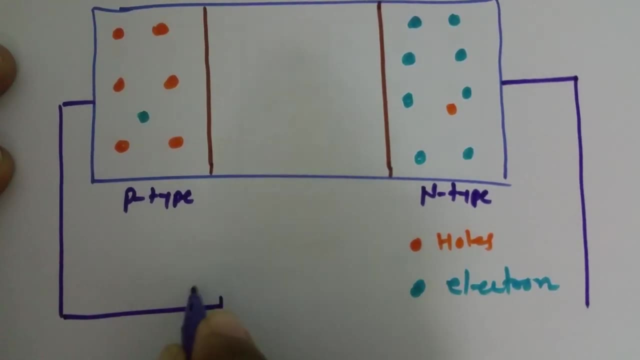 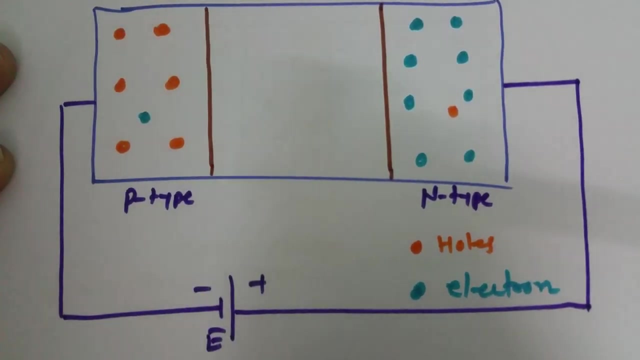 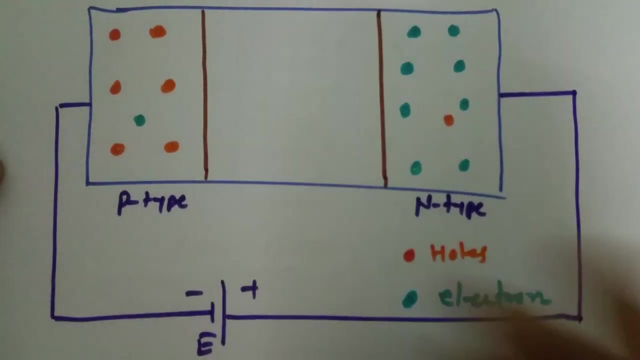 So let us connect that to battery in reverse bias. and to have reverse bias connection we need to connect p-type material with negative terminal of battery and n-type material to positive terminal of battery, So as if I connect this p-n junction in reverse bias, depletion region will increase. 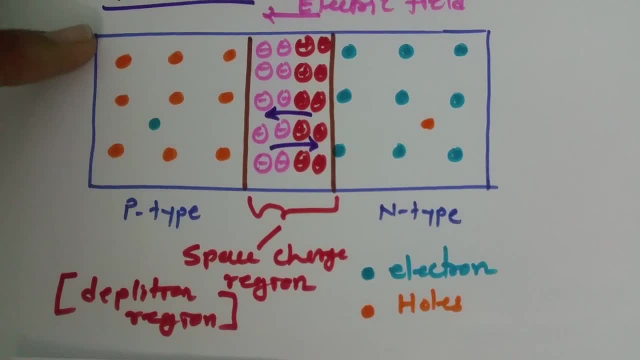 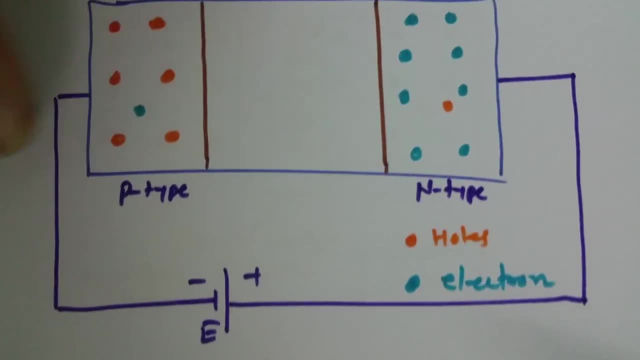 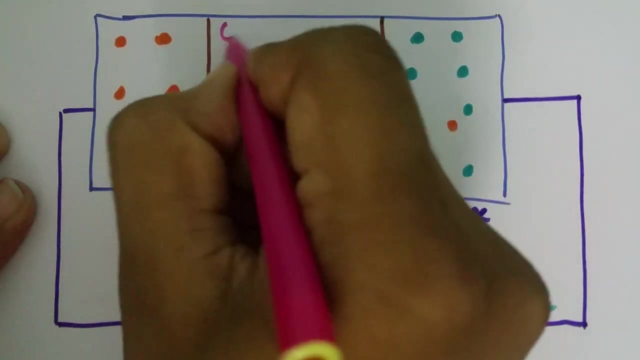 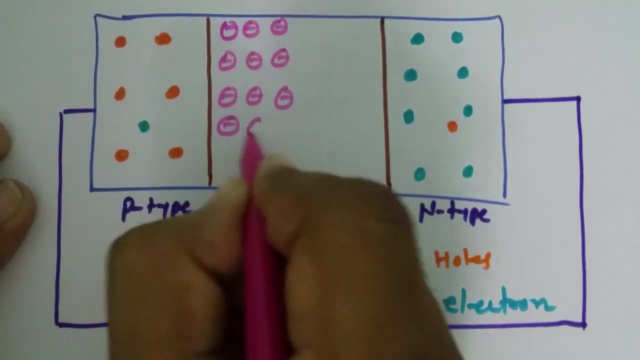 Now let us see this depletion region without any bias. So at that time we can observe depletion region width is this much, but after connecting this p-n junction in reverse bias depletion region is getting increased. So ultimately we can say this phase charge region that will be broad, which we can see. 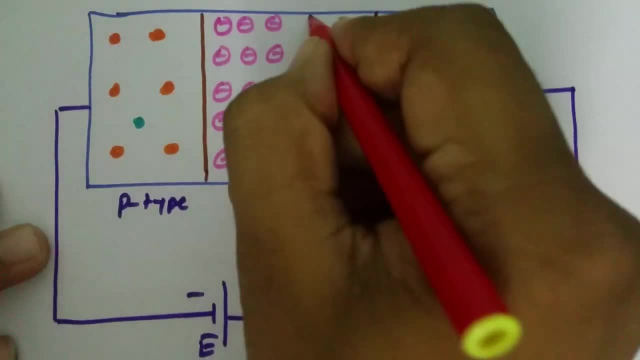 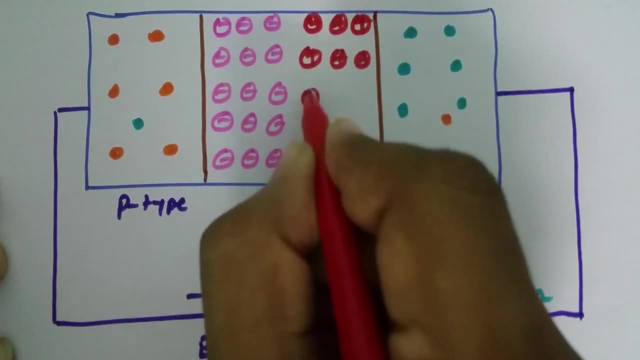 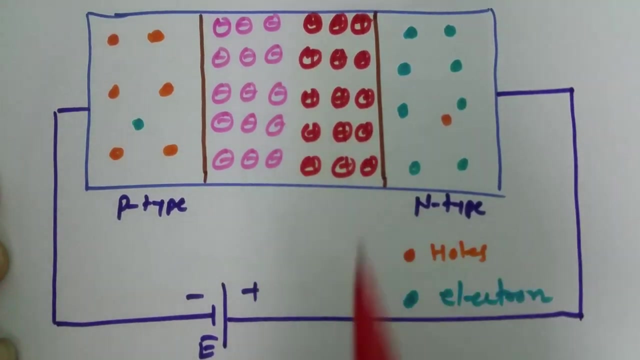 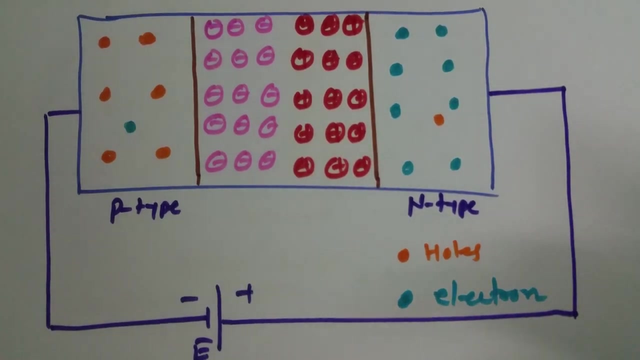 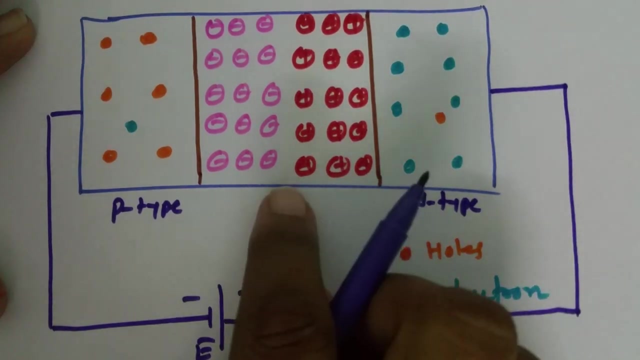 in this figure And positive charges that will be there at the side of n-type material. that is even getting broader. So this is how region is getting expanded. So here, as we increase reverse bias voltage, this depletion region will increase. So as this depletion region is increasing, this phase charge region will increase. 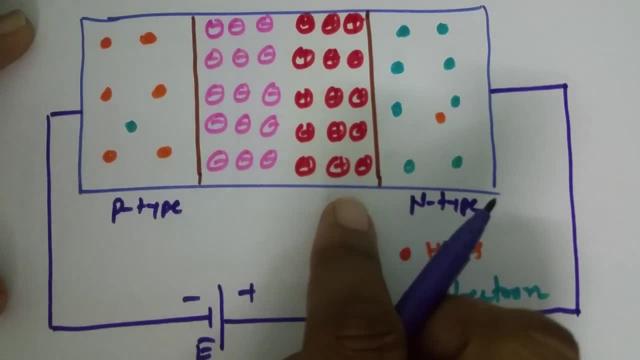 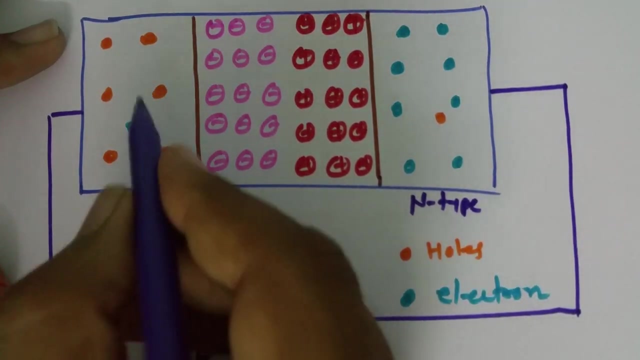 So this is the depletion region And very little. the charge being divided in this point, which is equal to this, is the gate that will. this is the gate that will beflow into the n-type material. Couldnot showae needle current getting deeper and deeper to dipize. 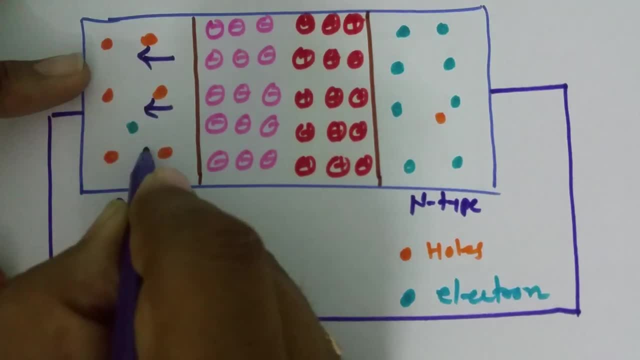 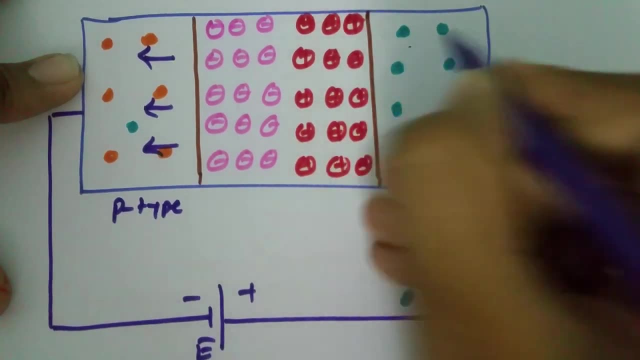 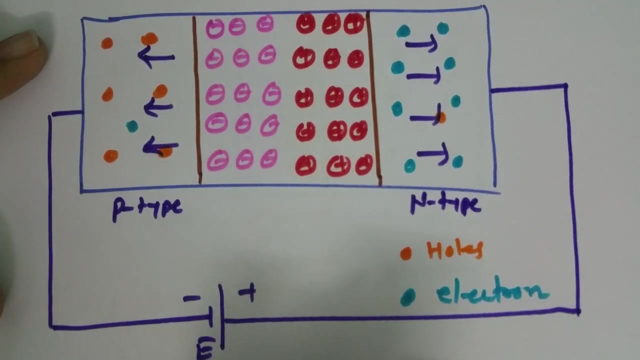 Now let us� allesiance this n-type material into y direction, And we'll move it. this way, electrons are getting pressure in this direction. So as we increase reverse bias voltage, this pressure is actually happening like this. So which is what? resulting into expansion. 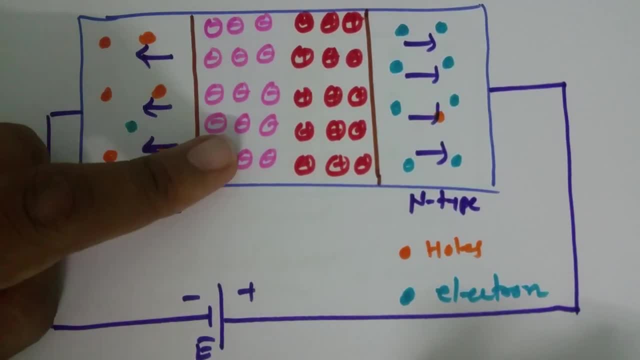 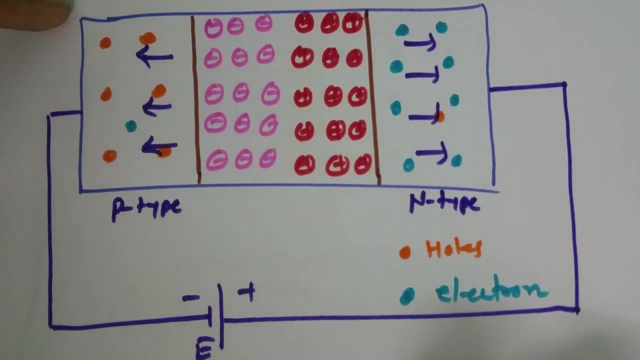 of depletion region and as we say, like, say, depletion region- width is more current- is not allowed to pass through that. but if we give more than the capacity of its sustainability, in that case this depletion region will get broken down and current will start to flow. 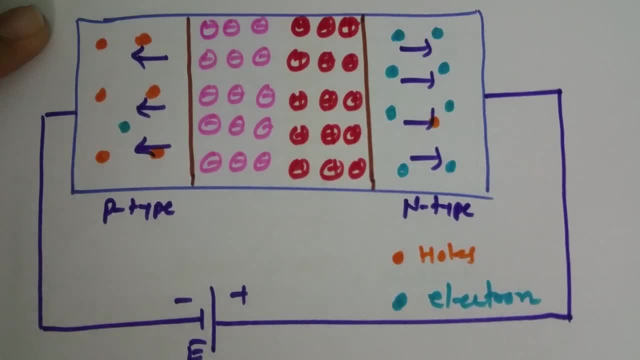 through that. So, after breakdown voltage, this p-n junction may get damaged and that is what, resulting into extreme high current flow in this direction, And that happens only if this breakdown of this junction is happening. So that is how reverse bias characteristic is there. So, basically, if we see how p-n junction functions, 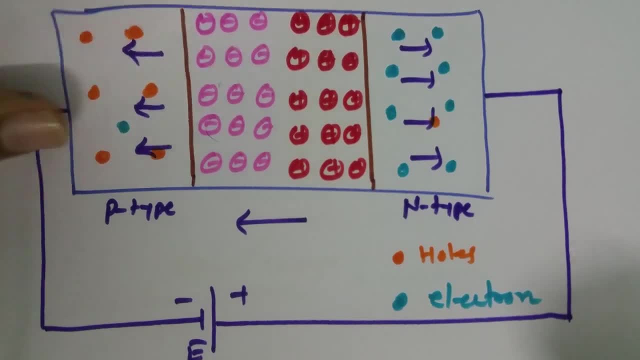 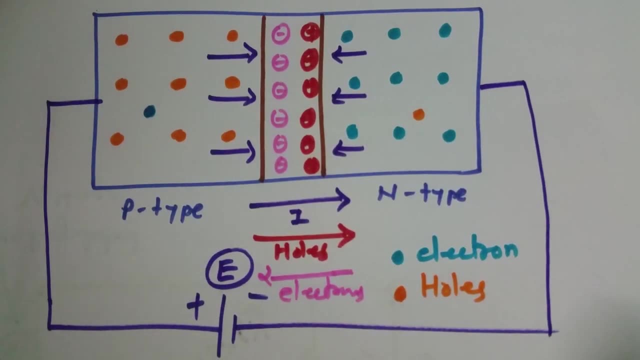 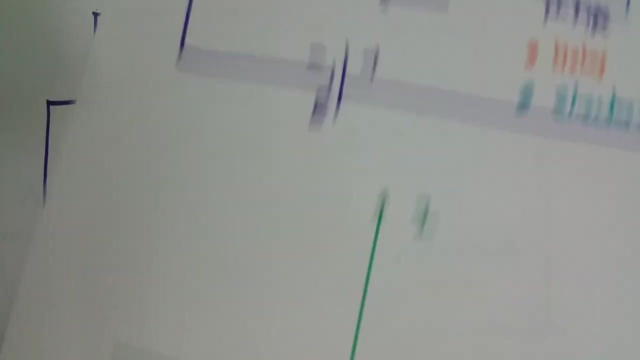 So p-n junction in forward bias functions as per: if we give voltage greater than potential barrier voltage, it will conduct from p type material to n type material And in this case in reverse bias, as if we give voltage greater than breakdown voltage, then only there will. 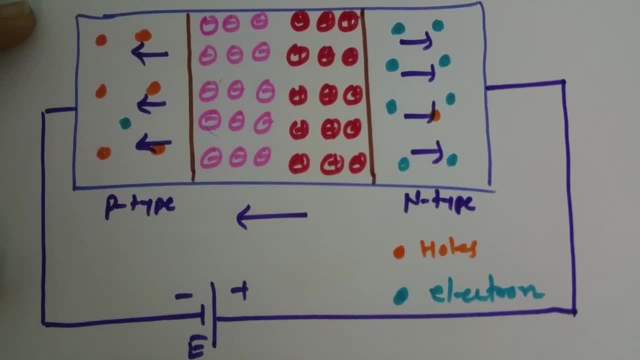 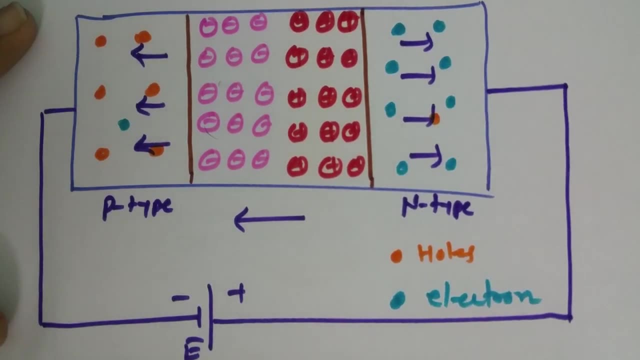 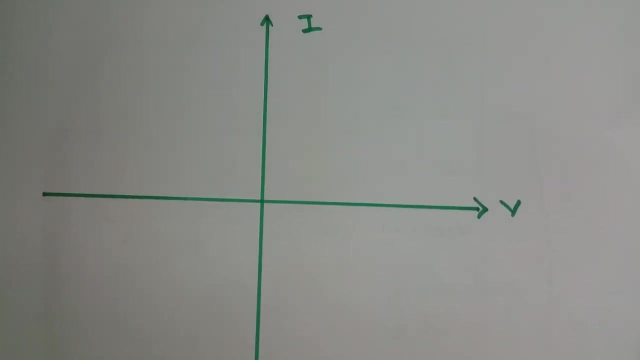 be a flow of current, Otherwise there will be a current which is there in terms of micro ampere, while if we conduct that p-n junction diode in forward bias, current will be peak. So here let us plot V-I characteristic of p-n junction diode. So if we see, this is 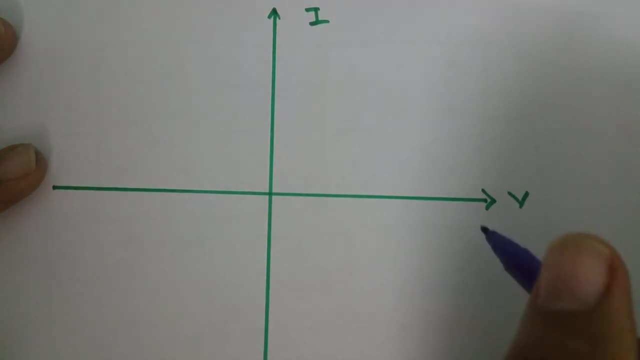 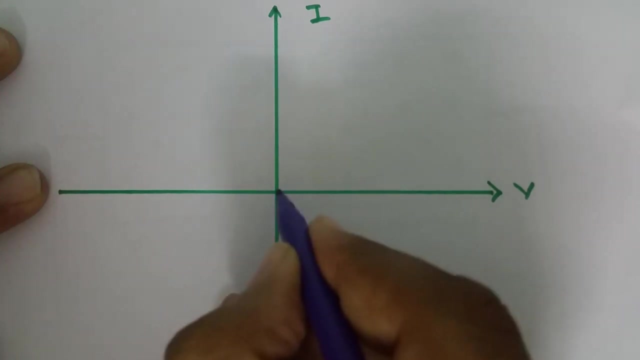 voltage and current. And if I keep anode positive with respect to cathode, in that case first quadrant, that will be forward bias characteristic. So initially if I increase voltage in forward bias there will be, there will be current, which is very narrow. but after, if I give voltage greater, 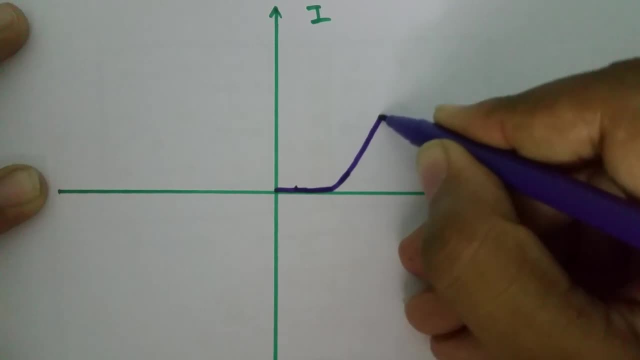 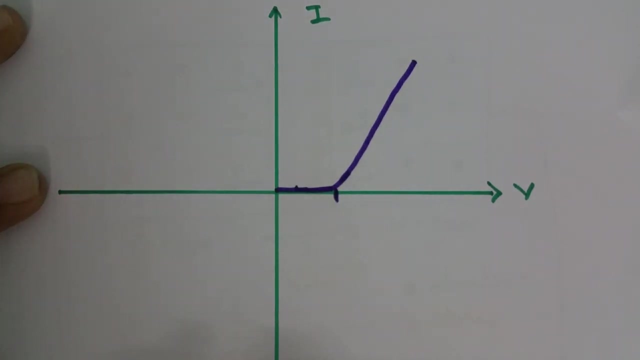 than potential barrier voltage, current will start to flow. So this is how characteristic will be there Now this voltage that is called as a voltage which is greater than potential barrier voltage. so that will be 0.7 voltage in case of silicon diode And in case of germanium p-n junction. 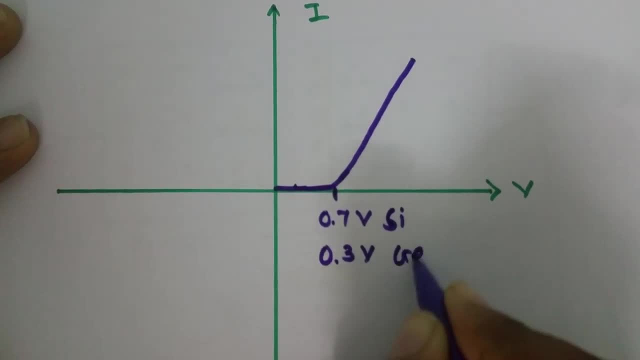 that voltage will be 0.3 voltage And as if I keep this p-n junction in reverse bias by giving positive terminal of battery to p-n junction, So if I keep this p-n junction in reverse bias by giving positive terminal of battery to p-n junction, then there will 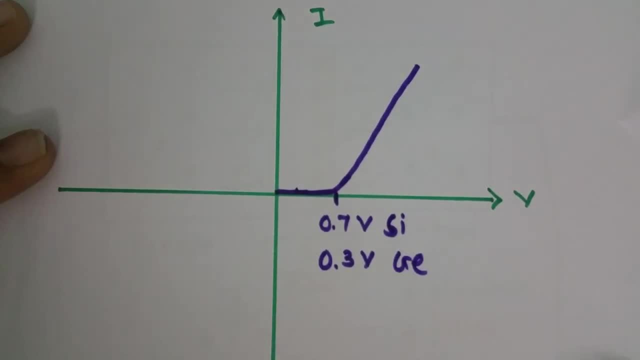 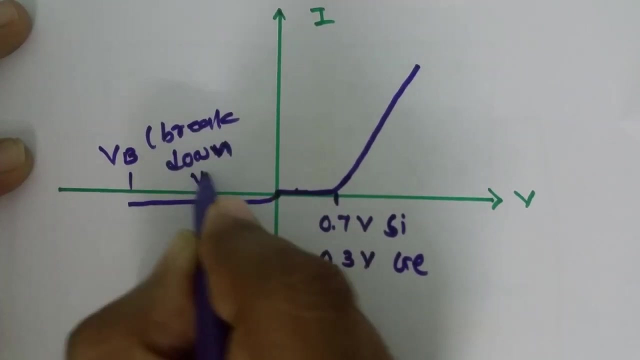 be 0.7 p-n junction in the second quadrant which I have shown the above, So we will have positive terminal of coke. So in this set of out- awesome, So we have 12 batteries- There will be negative terminals.